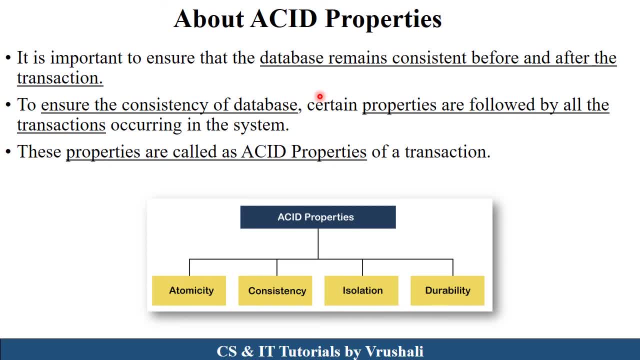 on the database, different transactions on the database. So at that time your database remains consistent. your database remains accurate before and after the transaction. That's why there are acid properties. this acid properties ensure that the consistency of database before and after the transaction. so all the transactions have follow this properties. so there are total. 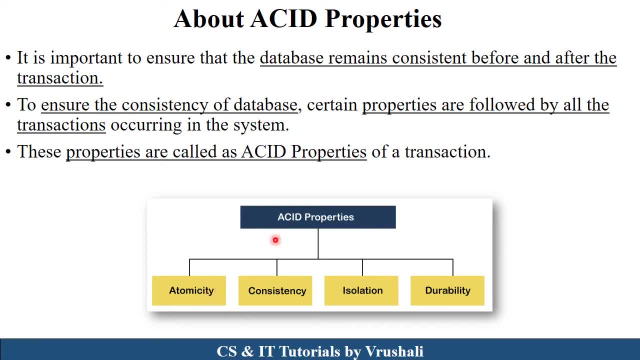 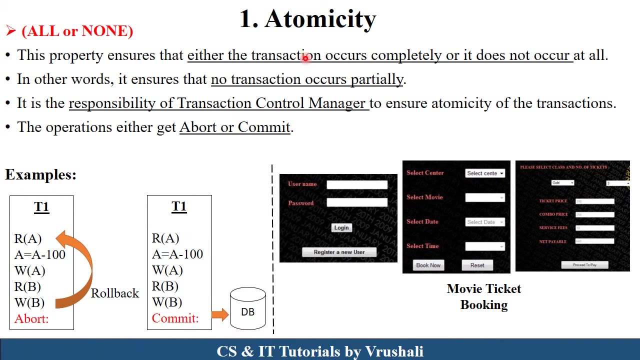 four acid properties here: A stands for atomicity, C stands for consistency, I stands for isolation and D stands for durability. if you follow all these acid properties, so your database always is in consistent state. there are no any errors or failures have occurred, right, that's why there are acid properties. next now, uh, this acid properties, or explain acid. 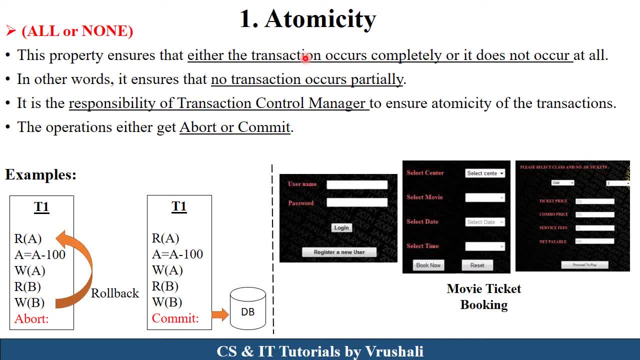 properties. this is one of the most important questions in your exam, so you need to explain all these properties with examples. so the first property is atomicity. while atomicity- you must remember this thing- either all transactions have performed or none of the transactions have performed. Okay, 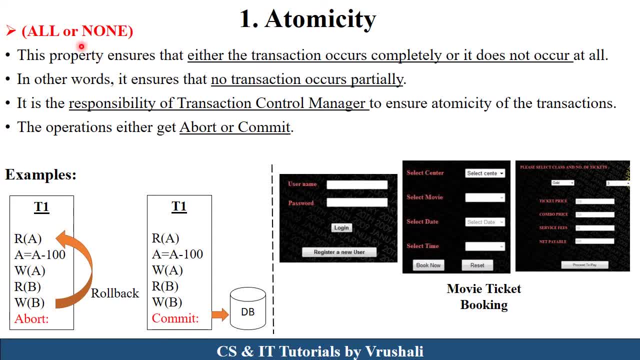 Okay, Okay, have performed. this is a rule of atomicity. right now, just focused here in this example, in this t1 transaction, cpu have performed different transaction right on the database, like read a, then a minus 100, write of a. after that they read b and write b. so while the performing the 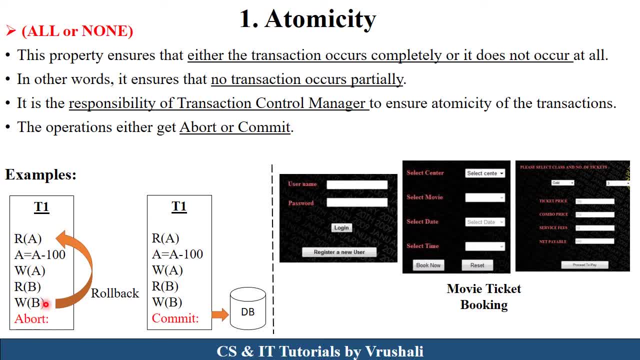 transaction. suppose some error have occurred before the commit statement. right, commit statement generally used to store all the data in database permanently. so before commit statement some errors have occur. so at that time this particular instruction or transaction get into the rollback state. rollback state means they again start from the first instruction. ok, so either this: 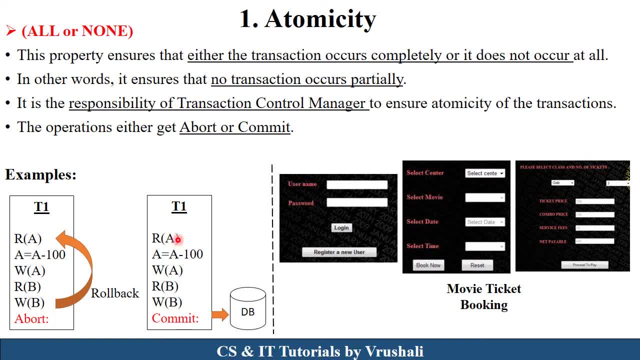 thing is happen in atomicity, or will you perform all the transaction and at the end, commit means all this data have stored permanently in database. so this is called as a atomicity: either transaction performed successfully on none of the transaction have performed, and this the response. 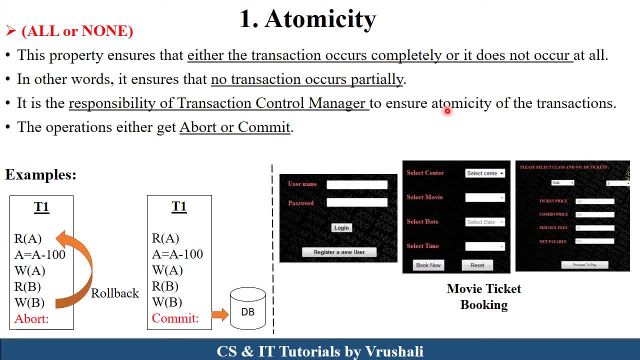 of transaction control manager. they ensure that atomicity of transaction. now let's see here some real-life example, that is movie ticket booking, when you book a particular ticket of the movie. so at that time first there is a login window, after that you select a movie, select a center, date, time and next when. 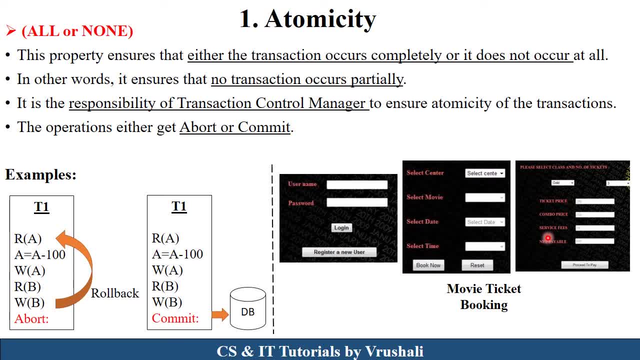 you go to next window for payment purpose. so some what? what happened? there are some server error or payment error. is there right? so at the time this is get into the rollback state means again you log in the system, again you fill the details right. so this is called as atomicity, either all the transaction. 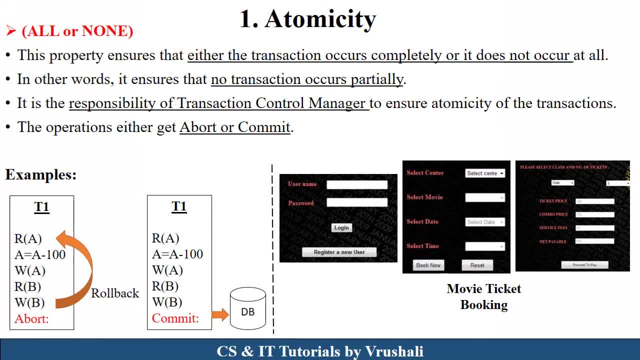 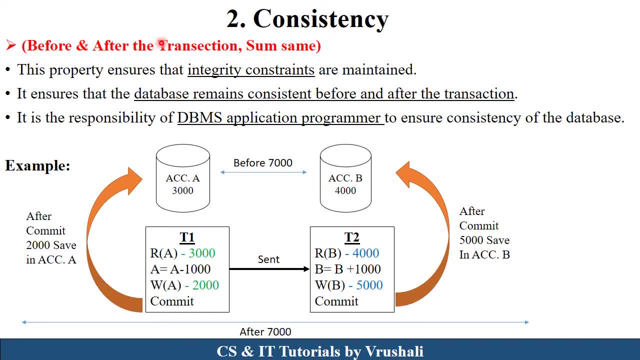 have performed and none of the transaction have performed clear. next, the next property is consistency. so consistency simply means before and after the transaction the value in database must be same. this is a called as consistency property. so this property ensure that integrity constraints. let's see how. now, just focused here on this 2 database, There is 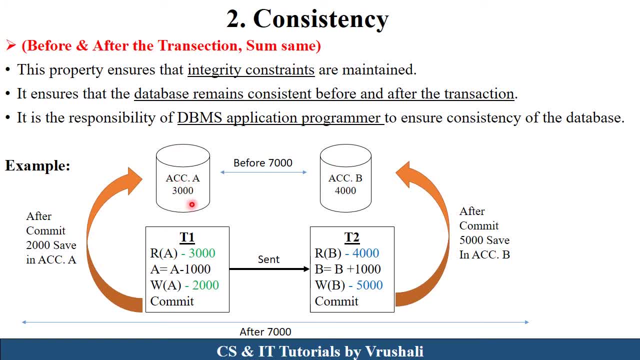 a four database. that is account a and in this account 3,000 rupees, and account B. having 4000 rupees means before transaction there are total 7000 rupees. right, this is your first step. in second step, see here: this is a T 1. 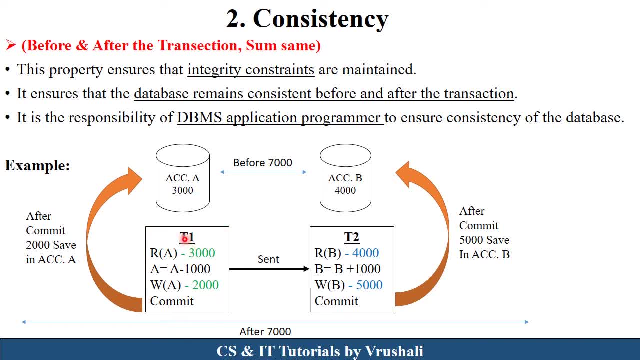 transaction. so what will? what was the approach of this T 1 transaction? they said: what was the T 1 transaction? if we decide to knead on, I don't have 7000 transaction? they say: what is your T 1 transaction if we decide to knead on? 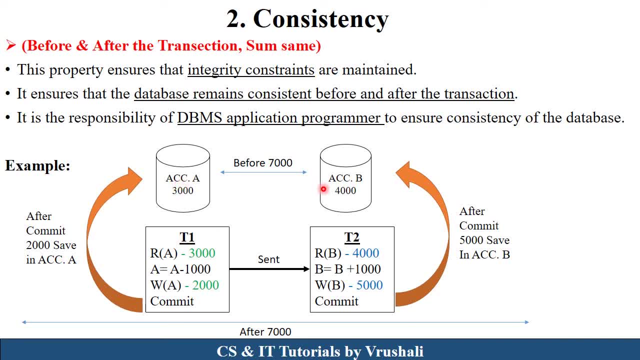 send 1000 rupees from account A to account B. okay, this is a problem statement. so first they read how much money in their account. so the read of A, read of A, means there are total 3000 rupees in the account. so A minus 1000. they send 1000 to account B or T2. so after sending 1000 they again 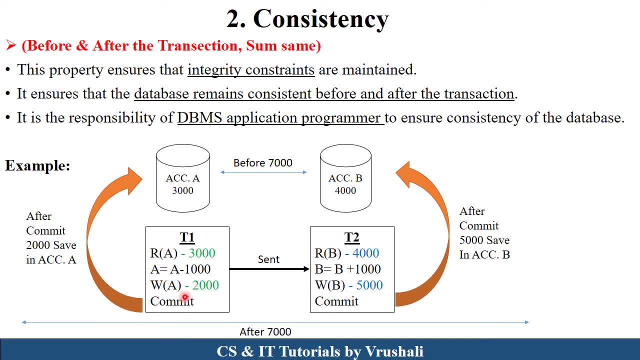 updated value into the database means write of A. so 2000 have stored into this account A now and commit means this transaction perform successful. now this 1000 send to T2 transaction now in this T2 first they read how much money in their account in the database. so read of B. 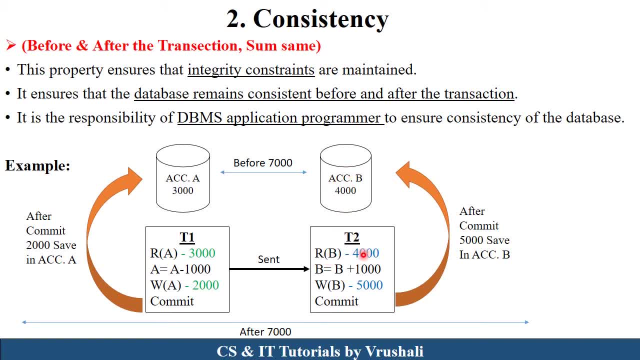 that is account P. so there are 4000 rupees before the transaction right. so B plus 1000. T1 send 1000 to T2. so B plus 1000 that is 5000. so write of B means this new value, that is 5000. have updated. 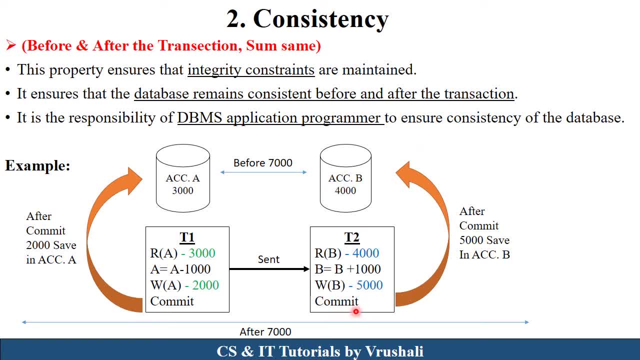 in this particular transaction. so write of B means this new value, that is, 5000. have updated particular database right and after that. commit means transaction have successful clear. so now after this transaction- see here, after the transaction in T1 there are how much rupees have remaining 2000 rupees because 1000 is sent to account B right. and after the transaction in T2: 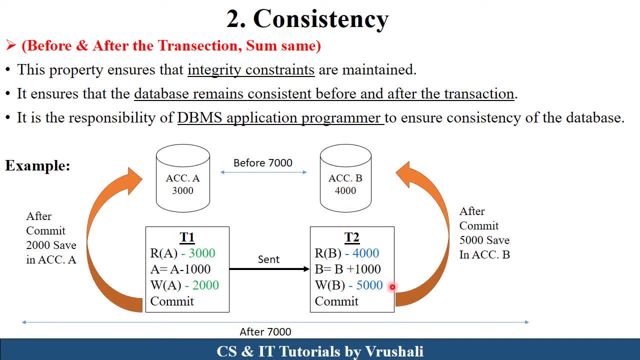 before 4000 rupees it gets 1000. so 4000 plus 1000, 5000 in this account right now. make the total before transaction 3000 plus 4000- 7000 rupees and after the transition here is 2000, 1000. send here account B. so 4000 plus 1000, 5000, right. 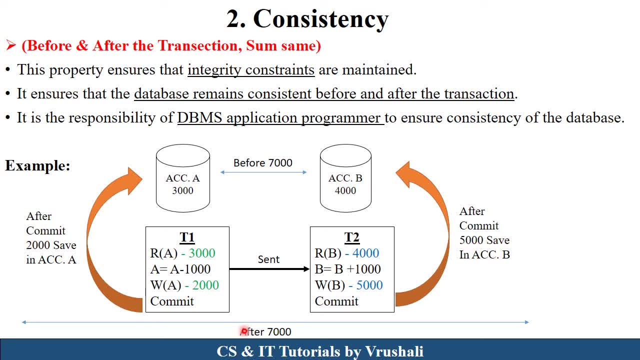 so 2000 and 5000 equal to 7000 right. so before transaction, 7000 rupees and after the transaction, 7000 rupees. this is called as consistency and this is the responsibility of DBMS application programmer. they handle this consistency of the database. right means before the transaction, 7000. 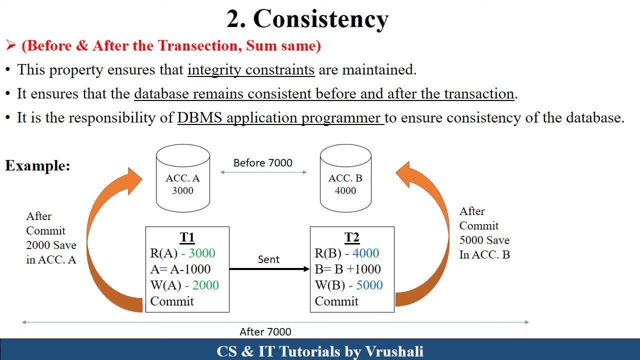 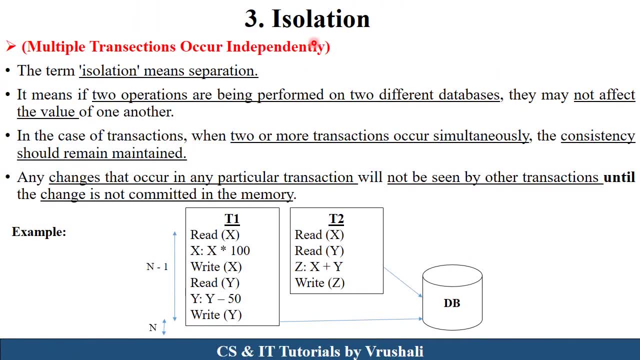 there is no any loss of information and no any loss of money. this is called as consistency. state clear next. the next is isolation, next, property. so isolation simply means you can perform multiple transaction independently on this same database. this is called as isolation. so isolation exactly means separation, means you can perform two or more transactions simultaneously on the database. 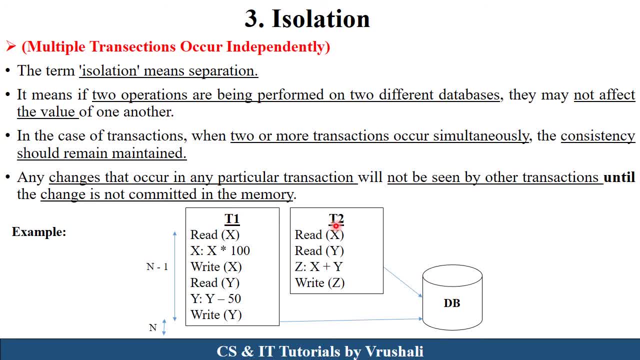 see here there is a t1 transaction and t2 transaction. so this transaction have performed on this database and this transaction have performed in database. right means any changes that occur in particular transaction will not be seen by other transaction. t1 doesn't know about t2. 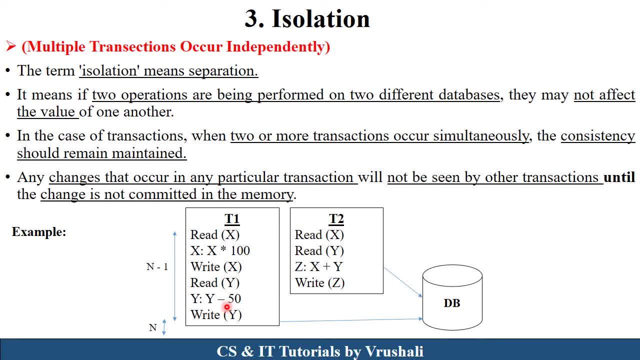 transaction. t2 doesn't know about t1. transaction means every transaction perform independently right on this same database. this is called as isolation, but this thing is happen until the change is not committed. okay, when t1 transaction mentioned the commit here, so at that time this data have.